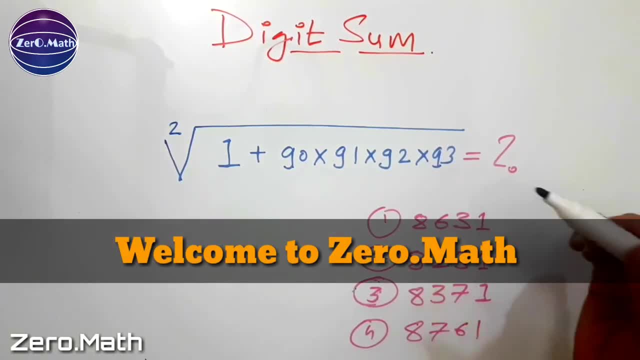 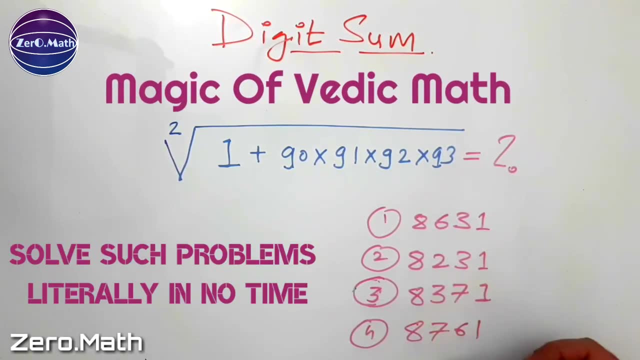 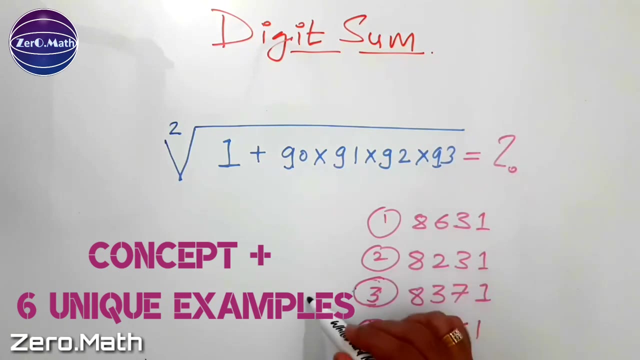 Hello friends, welcome to Zeromath. Today we are going to learn the magical concept of digit sum and its application to solve the complex mathematical problems like this. So after watching this video, you can solve such problem literally within no time. Let's learn how. 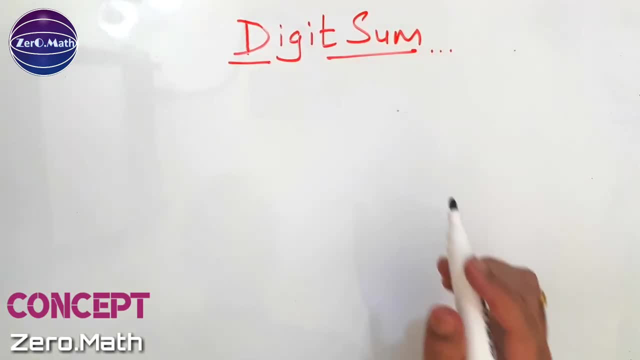 So, friends, let's first understand the concept of digit sum. So digit sum, as the name says, is a sum of digits of a number. So if I have a number 1,, 2 and 3, the digit sum of 1,, 2, 3 will be 1 plus 2 plus 3, equal to 6.. So 6 is a digit sum of 1,, 2, 3.. 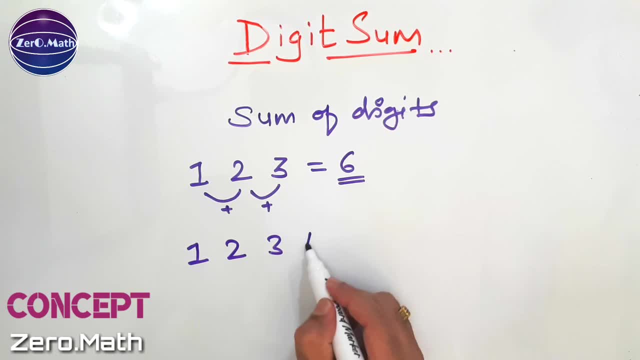 If I have a number: 1,, 2,, 3,, 4.. The digit sum will be 1 plus 2,, 3 plus 3,, 6 plus 4, 10.. However, please note, the digit sum cannot be a two digit number. Hence you have to add 1 and 0, which is equal to 1.. So digit sum of 1,, 2,, 3, 4 is 1.. So you have to keep adding till you get a single digit number. That's the concept of digit sum. 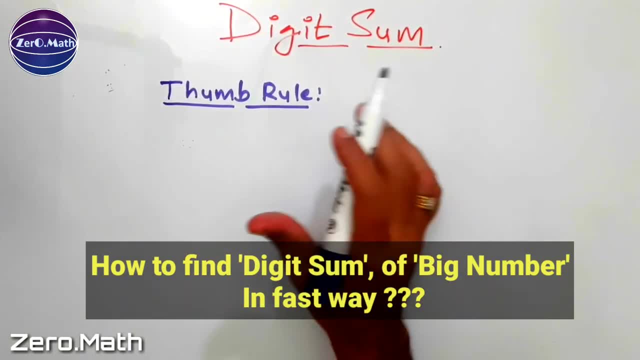 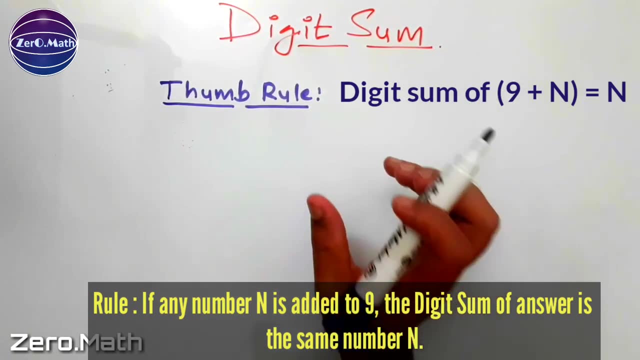 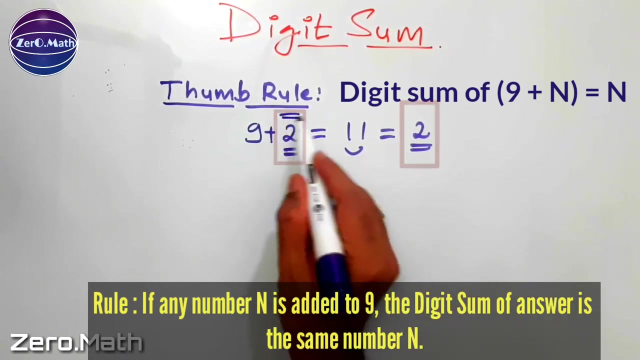 So, friends, let's understand the thumb rule to find out a digit sum of big numbers. So the rule is: if anything added to the number, it is a digit sum. So if I add 1 to the 9, the digit sum of the answer is always that number. For example, if I add 2 to the 9, I am going to get 11.. 1 plus 1 is equal to 2, which is my digit sum of the answer, which is equal to the same number which I added to 9.. 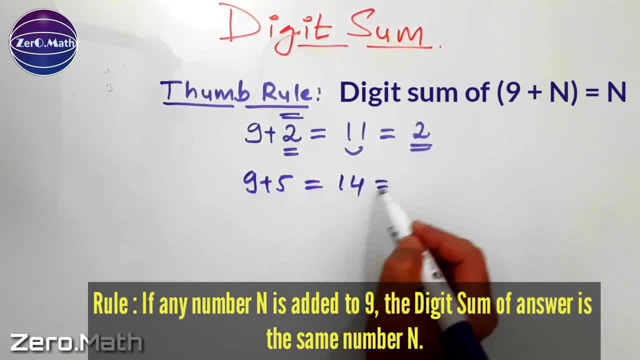 9 plus 5 is 14.. So digit sum of 14 is 4 plus 1, 5.. So if I add 5 to the 9,, the digit sum of answer is always 5.. Let's try to find out. 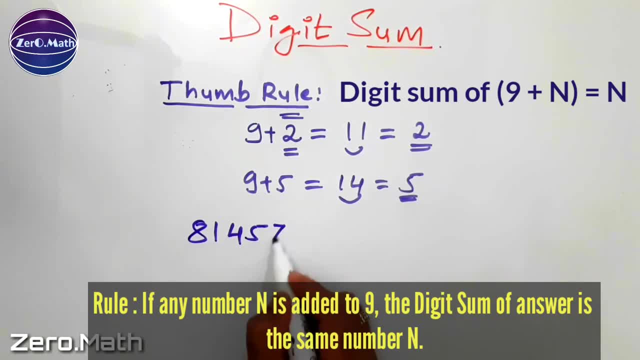 So the digit sum of 8,, 1,, 4,, 5,, 7.. So, using the normal method, what you will do? 8 plus 1,, 9,, 9 plus 4,, 13, plus 5,, 18, plus 7, 25.. 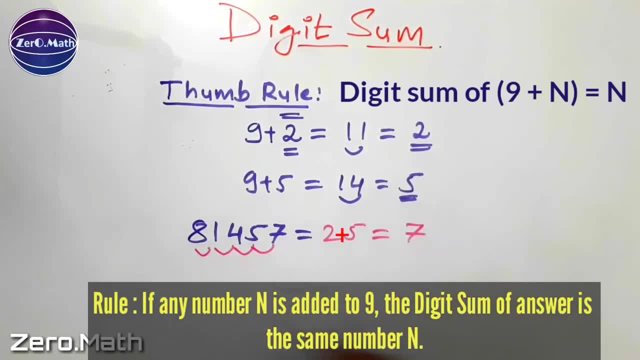 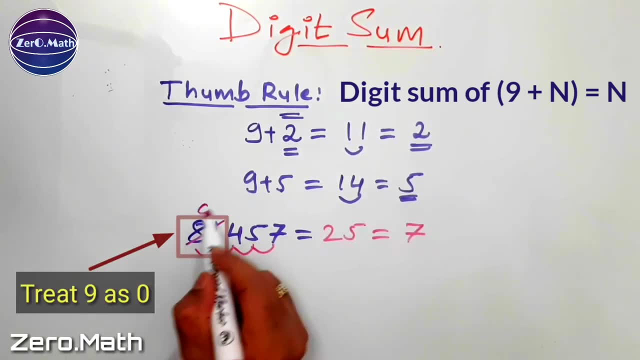 So the digit sum is 7.. However, no need to perform all this calculation The moment you will see 8 plus 1, 9, just cancel it out and treat it as 0. Because anything I add to 9,, I am going to get the same number. 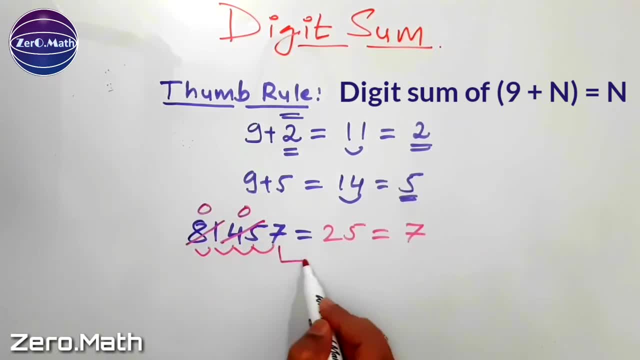 4 plus 5, 9,. treat it as 0.. So what I am going to get? 7,, which is my digit sum. Take one more example: 6, 3, 4, 4, 1, 0, 2.. 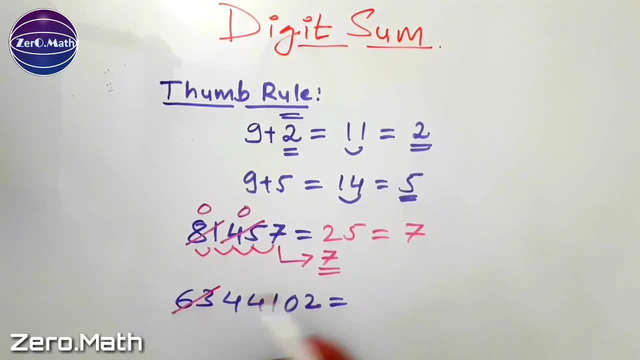 Find out the digit sum. So 6 plus 3 is 9,- treat it as 0.. 4 plus 4,, 8 plus 1,: 9, treat it as 0.. So what I am going to get? 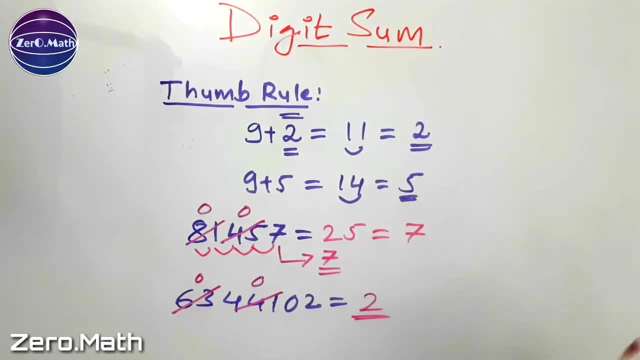 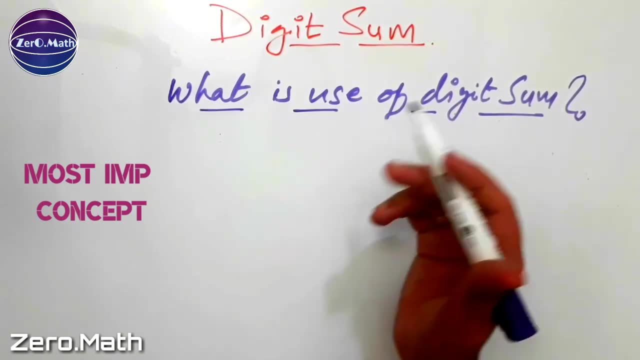 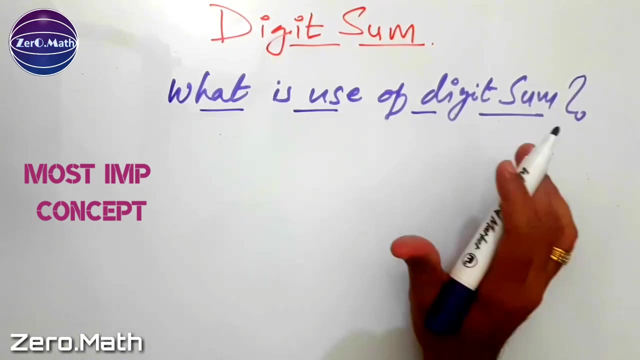 2,, which is my digit sum. See how easy it is. So you will say: we will learn What is digit sum. How do you calculate digit sum? But what next? What is the use of digit sum? Let's understand the application of digit sum. 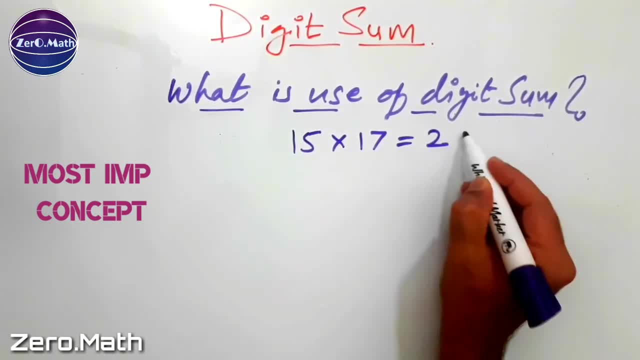 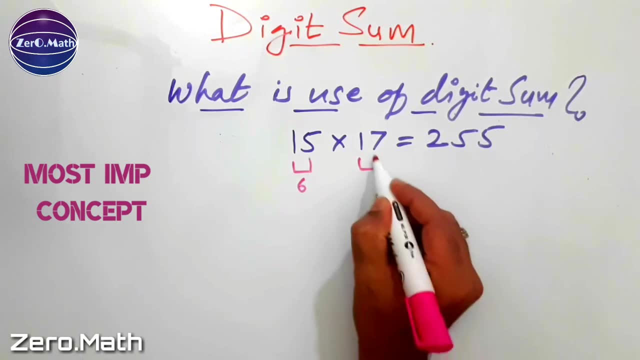 Let's take one example: 15 into 17 is equal to 255.. Let's find out the digit sum of left hand side: 5 plus 1 is 6.. 7 plus 1 is 8.. 6 into 8 is 48.. 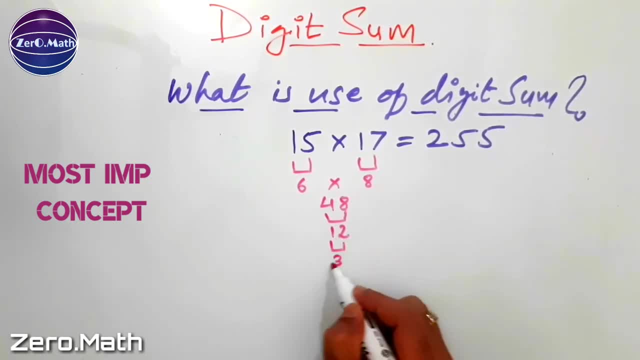 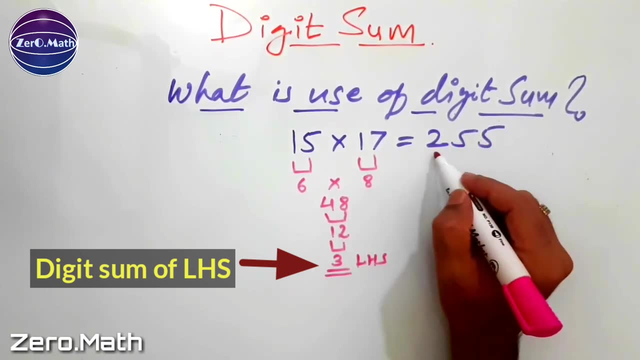 8 plus 4 is equal to 12.. 2 plus 1 is 3.. So 3 is the digit sum of left hand side. Now calculate the digit sum of right hand side: 2 plus 5 is 7.. 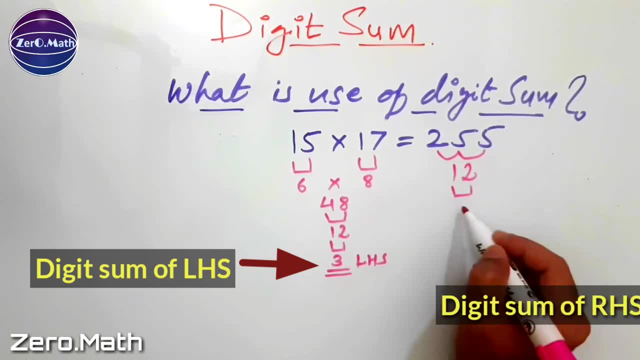 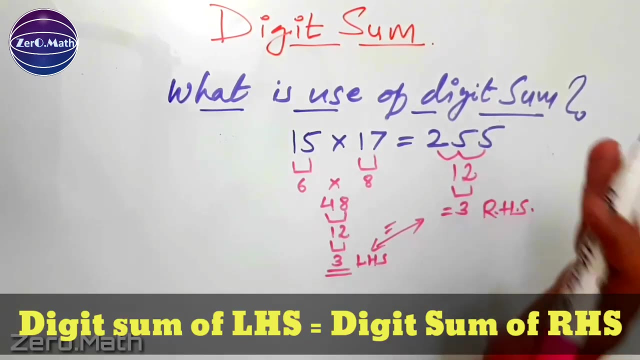 Plus 5 is 12.. 1 plus 2 is 3, which is the digit sum of right hand side. So you can see, the digit sum of left hand side is always equal to the digit sum of right hand side And there is a thumb rule which you should remember. 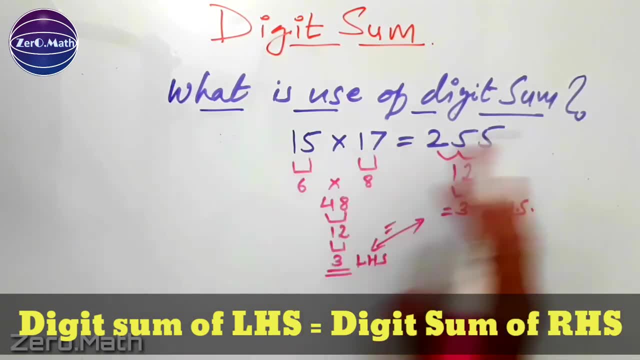 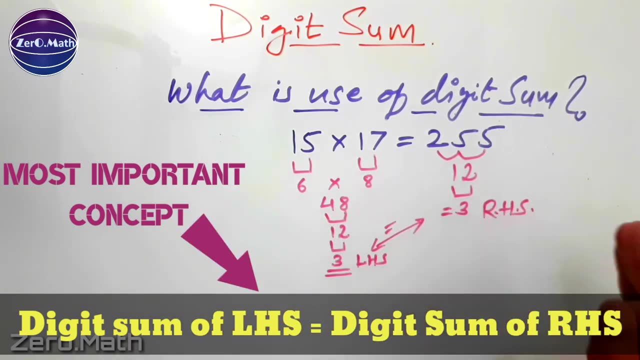 In any competitive exam, when you will get any complicated problem, the digit sum of the left hand side and right hand side is going to be always the same. This is the most beautiful mathematical equation which is going to save you a lot of time in any competitive exam. 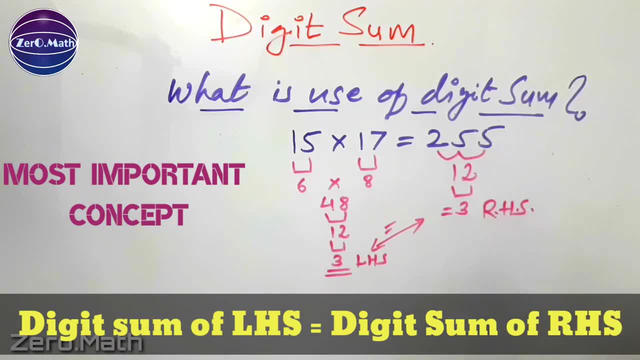 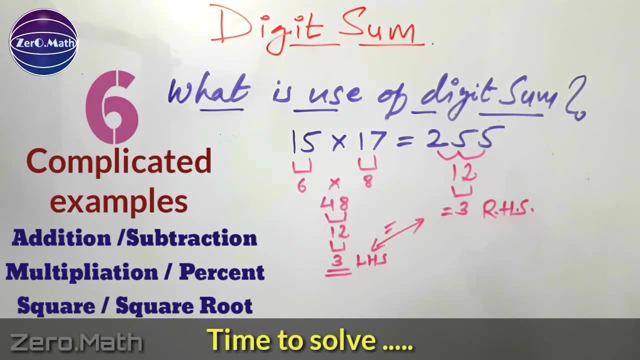 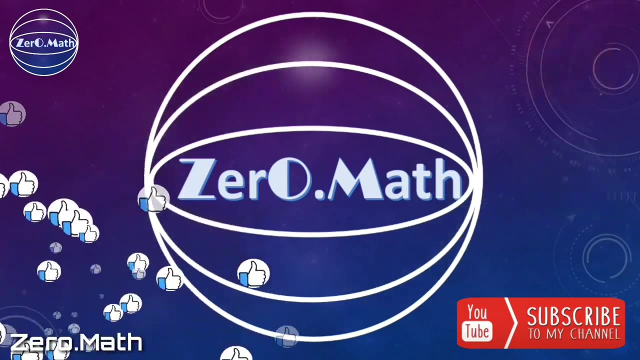 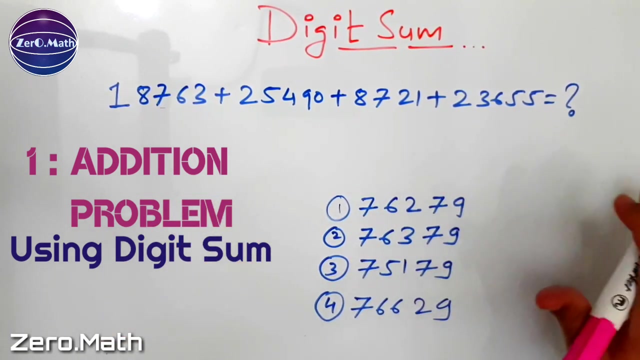 So, friends, let's move on to some examples, in fact the complicated examples, which we will try to solve using the digit sum method. Friends, we are going to solve various problems of addition, division, multiplication, square, square root, using the digit sum method. 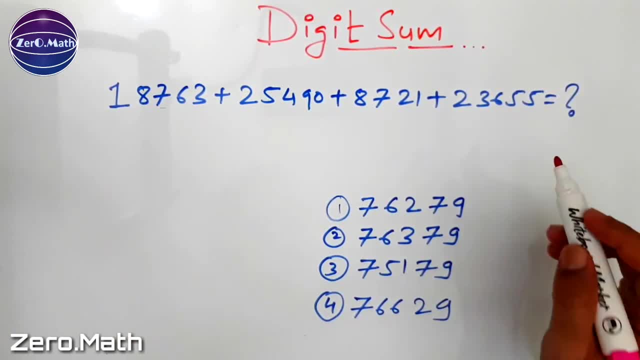 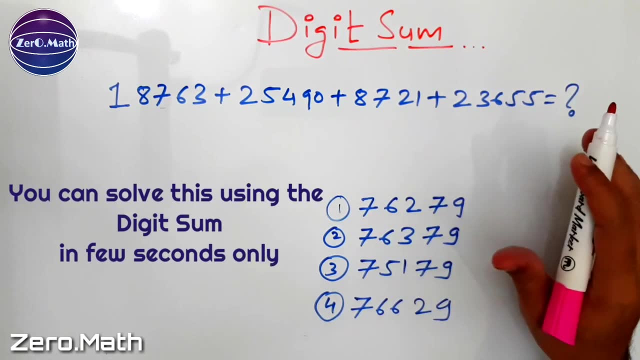 Have a look at this addition problem. If you try to solve this problem with pen and paper, it is at least going to take 40 to 50 seconds for you, even if you are very good at calculation. Also, you can look at the options. 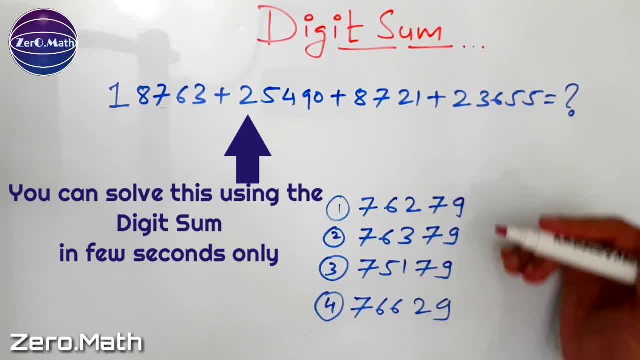 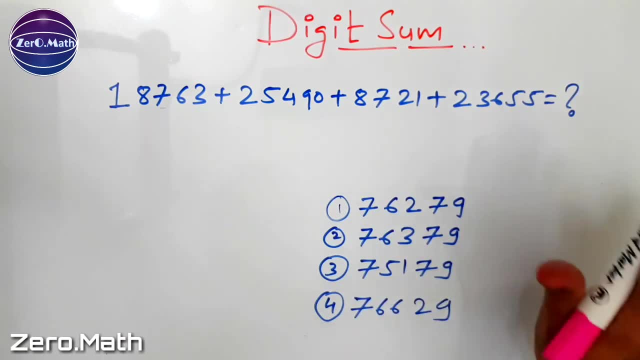 The options are also very close, So you can look at the options. So in exam you cannot really judge the answer very easily. Let's solve this problem using the digit sum method. So, as per our concept of digit sum, digit sum of left hand side is equal to digit sum of right hand side. 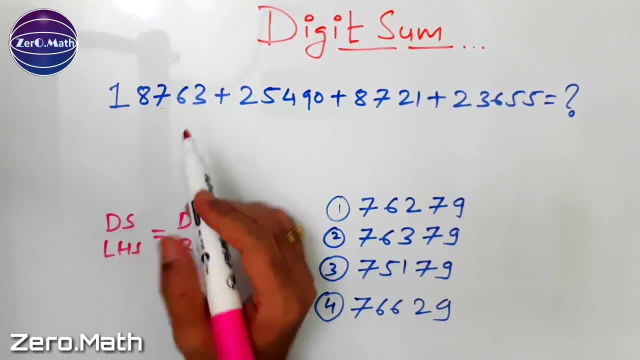 So let's find out what is the digit sum of left hand side. So on left hand side, 8 plus 1 is 9.. So we treat it as 0.. 6 plus 3 is 9.. Again, it is. 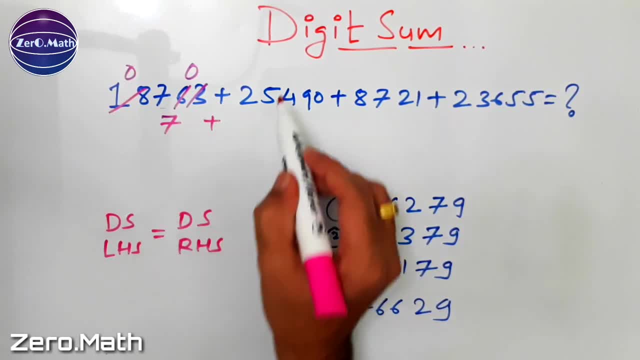 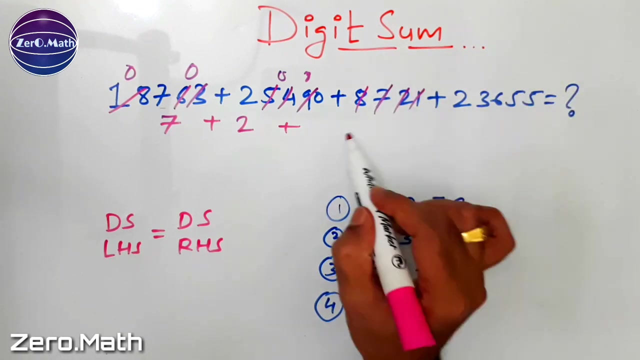 So it is, the sum will be 7 here plus 5 plus 4, 9,, which means 0, 9 is 0. So the digit sum is 2 plus find out the sum of 8, 7, 2, 1, 8 and 1, 9, 1, 7,, 2, 9,, which means it is also 0 plus 2, 3, 6,, 5, 5.. 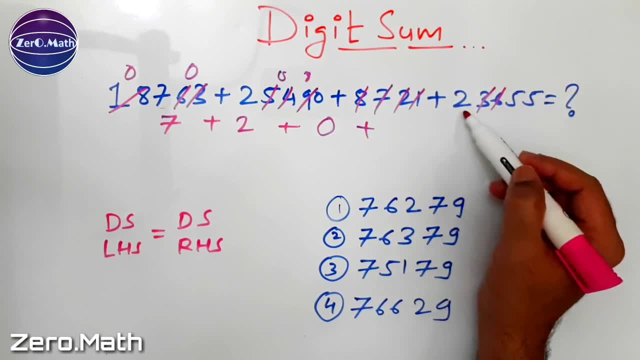 So 6 plus 3,, 9,, which is 0,, 5,, 5,, 10 plus 2, 12.. So 12 means 2 plus 1 is equal to 3.. So digit sum is 3.. 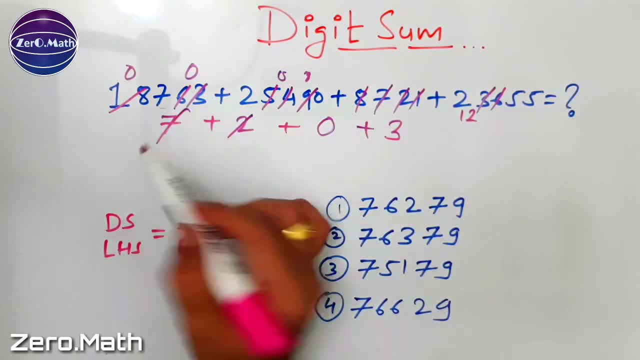 So find out the digit sum again now: 7 plus 2, 9.. So 9 means 0. So the digit sum will be 3.. So digit sum of left hand side is equal to 3.. Hence the digit sum of right hand side has to be 3.. 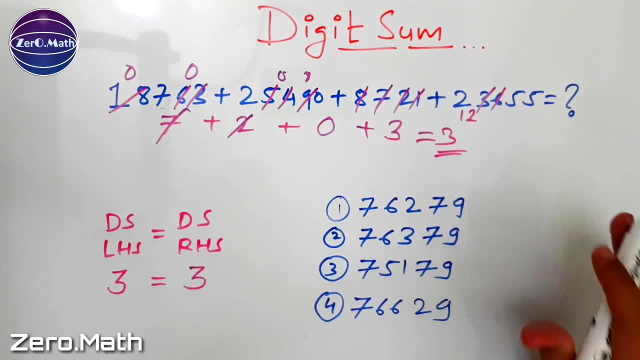 So let's figure out out of this 4 option which option's digit sum is 3.. So take the first option. So here 9 gone, which is 0, 7 plus 2, 9, which means it is also 0. 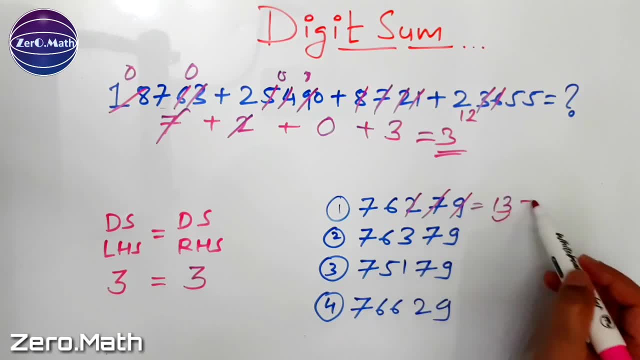 So 7 plus 6 is 13.. So 1 plus 3 is equal to 4,, which is not equal to 3,, then which means this cannot be my answer. Let's take the another option, option 2.. So this 9 means 0, 6 plus 3, 9 means 0, 7 plus 7, 14.. 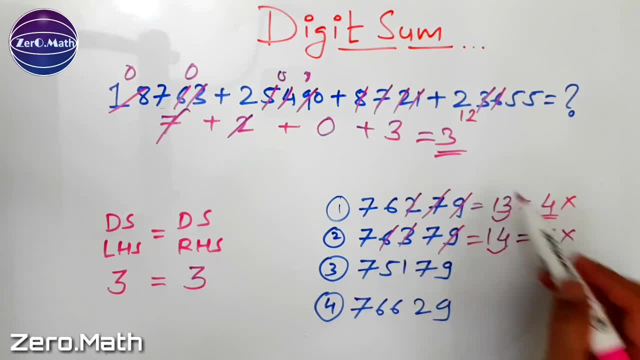 So 1 plus 4 is equal to 5,, which cannot be our answer. Move to the third option. So 9 gone, this 7, 7, 14.. Plus 5 plus 1, 6.. So 14 plus 6 is 20.. 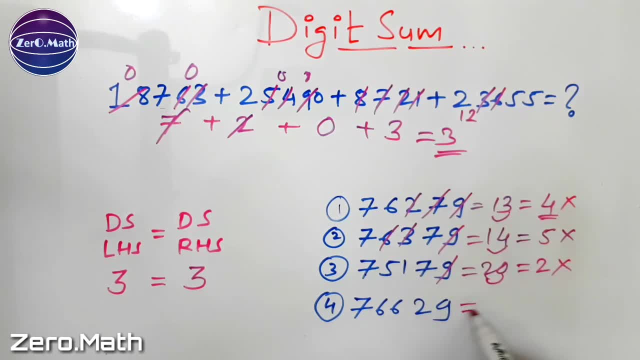 So 20 means 2 plus 0 is 2,, which cannot be our option. So let's look at option 4.. So this 9 means 0, 7 plus 2, 9 means 0, 6 is 12.. 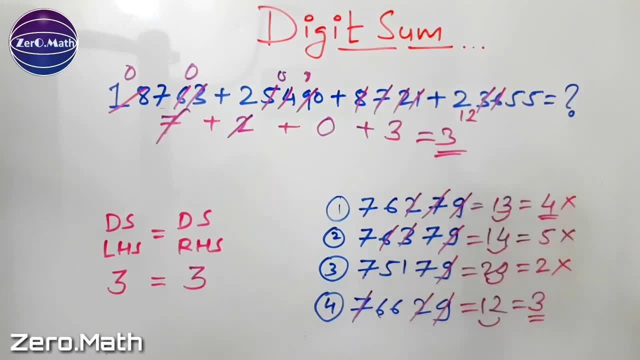 2 plus 1 is equal to 3, which is equal to. yes, what is the digit sum of left hand side? So which means the correct option is option 4.. So you can see how easily we crack the correct option. 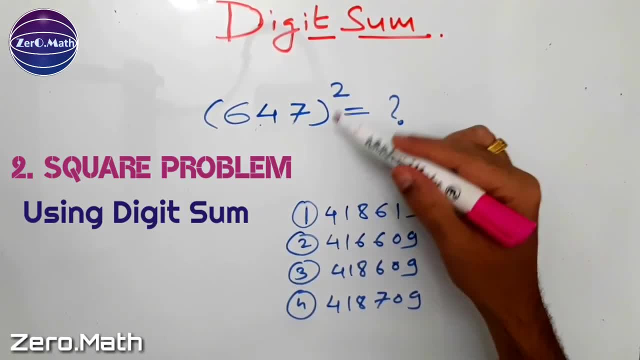 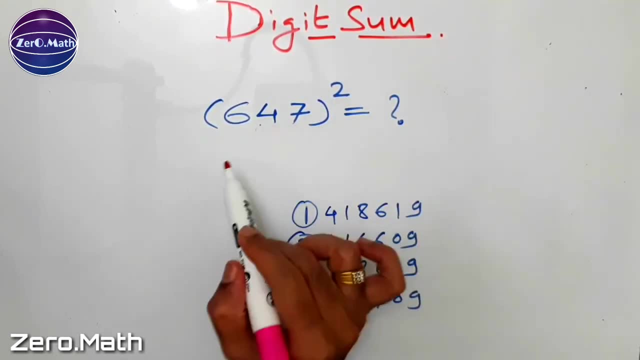 Let's solve this square problem using the digit sum method. So square is nothing but multiplication: It's 647 into 647.. So let's take digit sum of left hand side, So 6 plus 4, 10 plus 7, 17.. 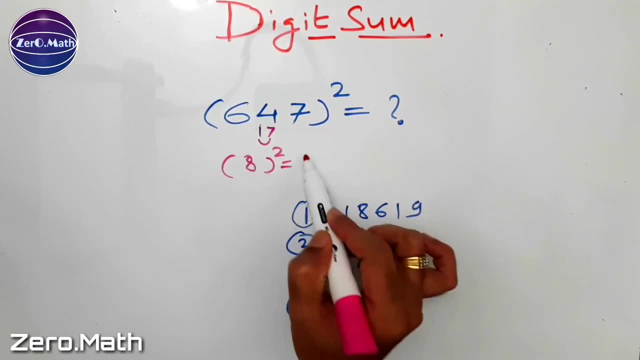 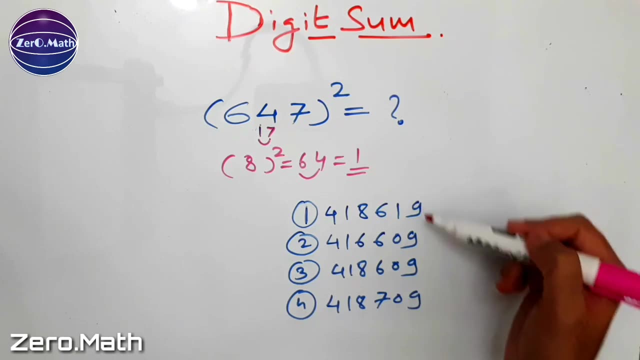 So 7 plus 1 is 8.. Let's square 8 is 64.. 6 plus 4, 10 is equal to, so digit sum is 1.. Let's find out out of this 4 option. which option has digit sum as 1.. 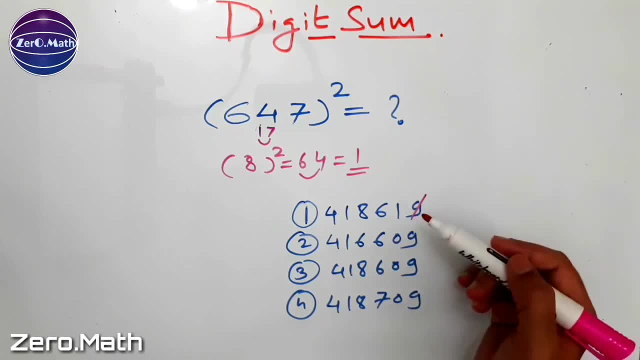 So take option 1, so this 9 gone, it is 0, 8 and 1, again 9.. So it will be 0, 6 plus 1, 7 plus 4, 11.. So 1 plus 1, 2,. this cannot be my answer. 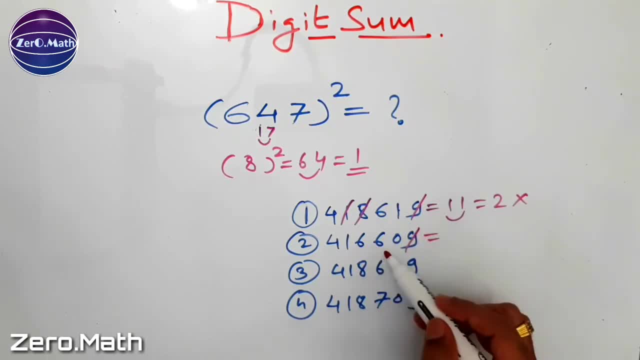 Digit sum has to be 1.. So take second option: 9 gone, 6, 6,, 12,, 1,, 13 and 4, 17.. So 7 plus 1, 8.. This cannot be my answer. 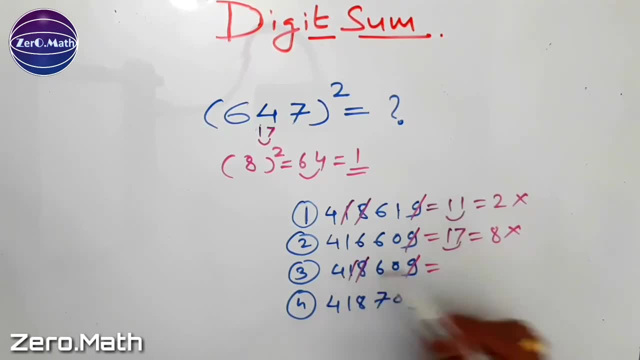 Take the third one: 9 gone 8 and 1, 9, again gone, 6 plus 4, 10.. 1 plus 0, 1.. So, yes, This can be my answer. Let's verify option 4 as well. 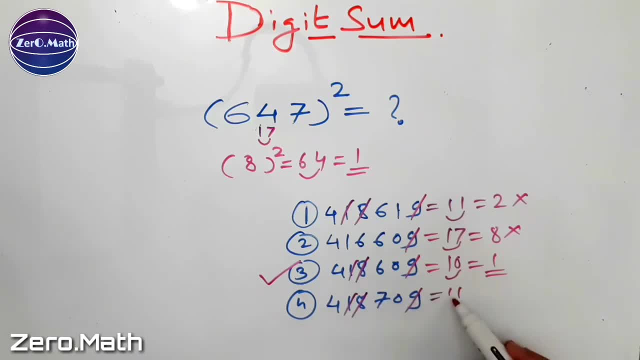 9 gone, 8, 1, 9 gone, 7 plus 4, 11.. 1 plus 1, 2.. So this cannot be my answer. So you can see how easily we cracked the answer. Let's solve this percentage problem and find out the value of x. 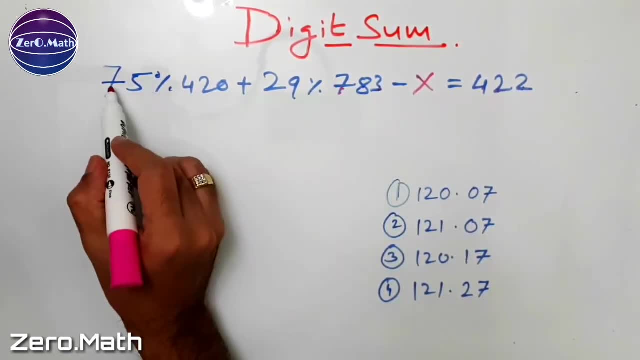 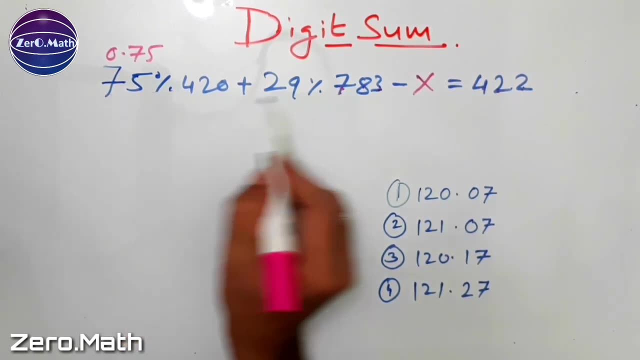 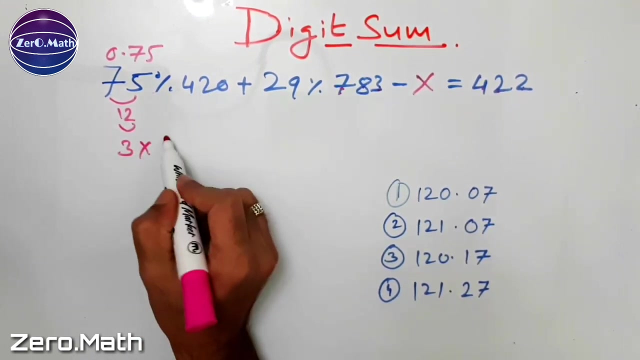 So the percentage means multiplication. When I say 75%, it is nothing but 0.75.. So it's as good as multiplication. Let's find out the digit sum of left hand side. So 75 is 7 plus 5 is 12, 2 plus 1, 3 into 4 plus 2, 6.. 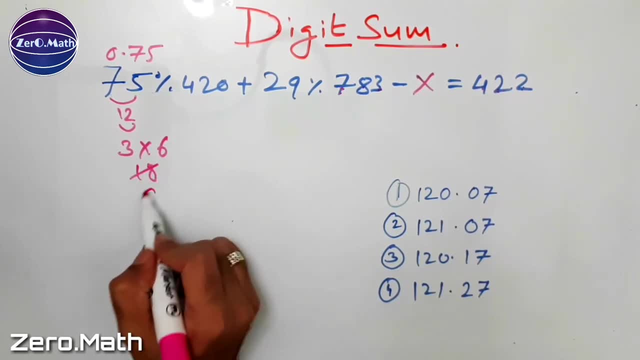 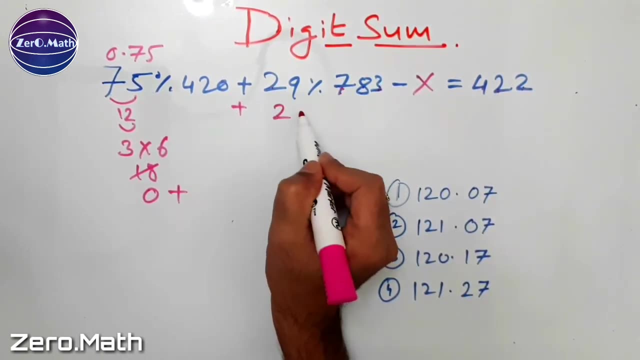 6 into 3 is 18.. So 8 plus 1 is 9.. So this will become 0. Plus. so let's find out the digit sum here: 9 plus 2, 11.. And 1 plus 1 is 2 into 7,, 3,, 10,, 8,, 18.. 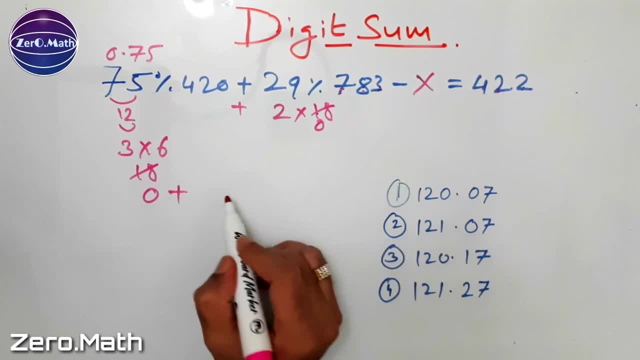 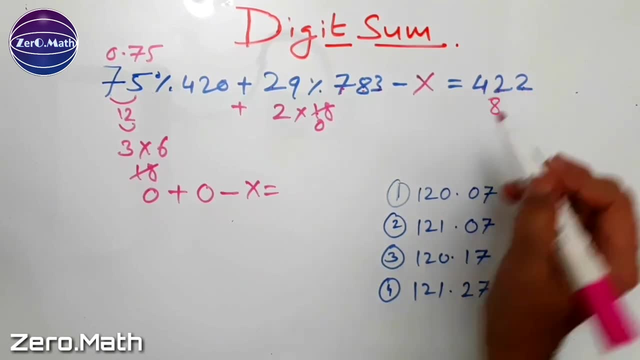 So 18 is again 8 plus 1, 9.. So 9 is nothing but 0.. So 0 into 2 is 0.. So minus this x is equal to 422.. 4 plus 2,, 6 plus 2, 8.. 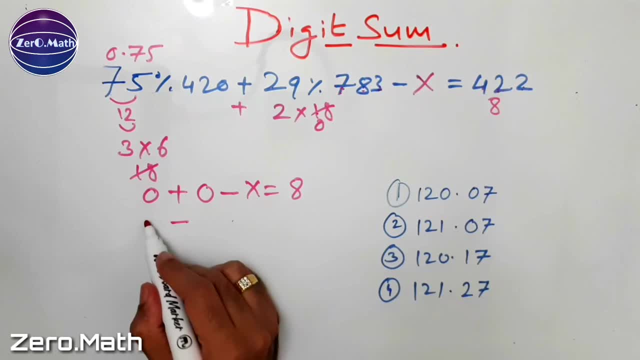 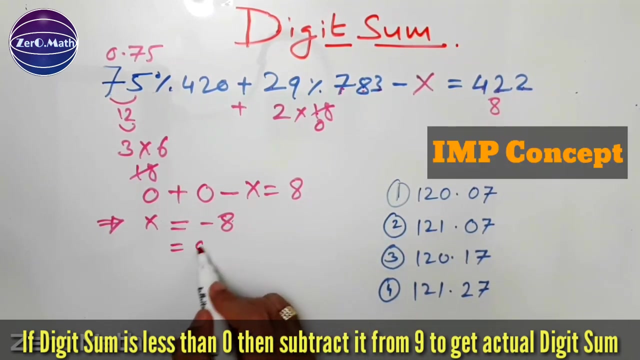 So digit sum is 8.. So here minus x is equal to 8. Hence x is equal to minus 8.. This is bit tricky and very important concept You have to remember whenever you will find a digit sum as negative value. what you are going to do? you simply subtract it from 9.. 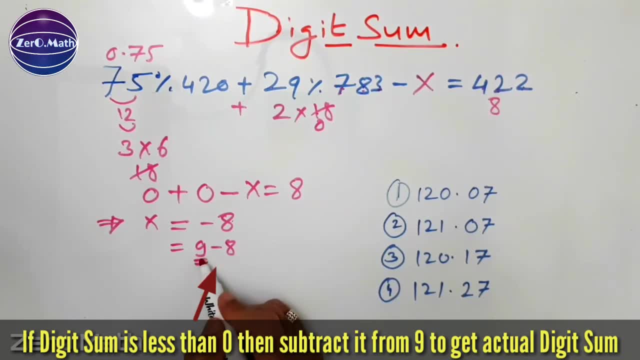 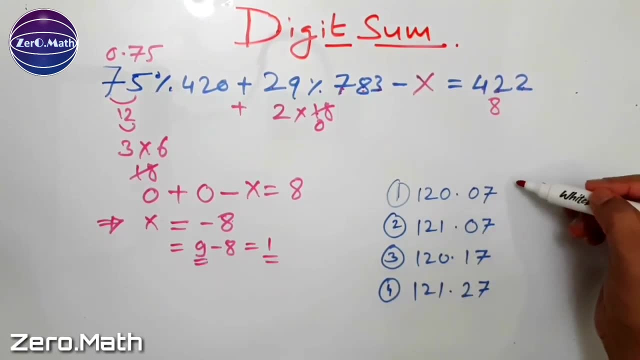 So you make it as 9 minus 8.. This is very important concept which you have to remember. So 9 minus 8 is equal to 1. So digit sum of this x is equal to 1.. So basically, what we are going to do out of this 4 option. 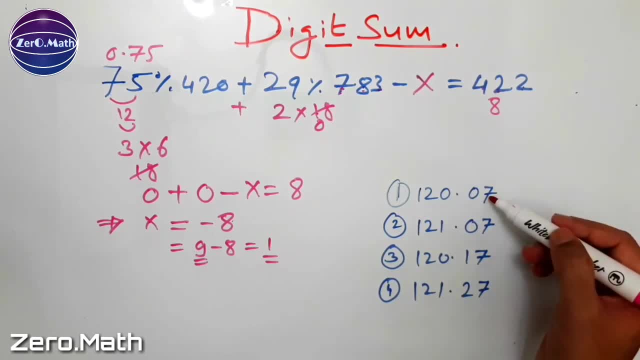 which option has digit sum as 1,? that is going to be my answer. So let's try option 1,, 7 to 9, which is 0.. So what is the meaning? 1.. My digit sum is 1.. 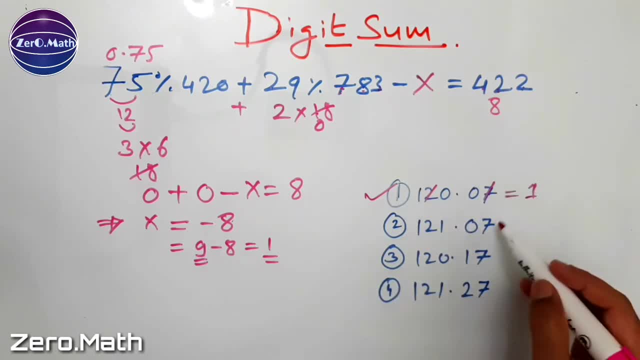 So yes, this is going to be my answer. Let's verify other 3 options as well. So 7 to 9 gone, 1 plus 1 is equal to 2.. This cannot be my answer. 7 to 9, so 1 plus 1 is 2.. 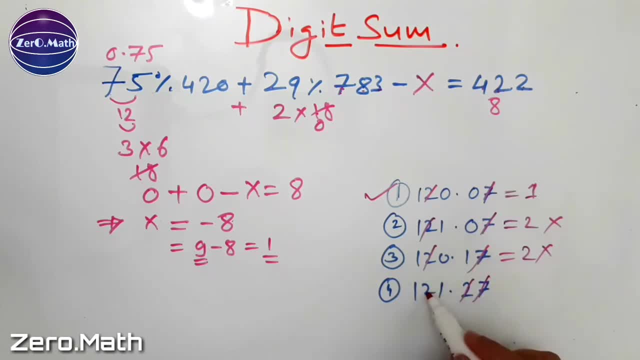 This cannot be my answer. So 7 to 9 gone: 2, 1, 3,, 1, 4.. This cannot be my answer, So the correct option is option 1.. So, friends, you can see this is a bit complicated problem. 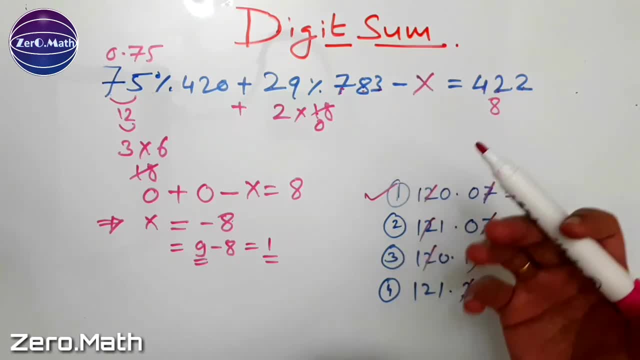 And in examination. they really don't expect you to do all this calculation. They know you are capable of doing calculation. What you have to do, you have to just figure out what is the correct option as fast as possible. Let's solve this division problem by the digitization. 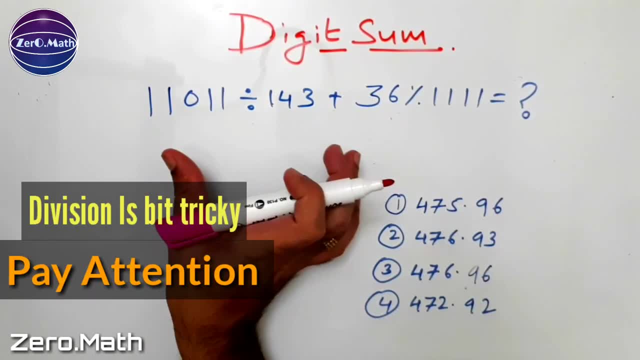 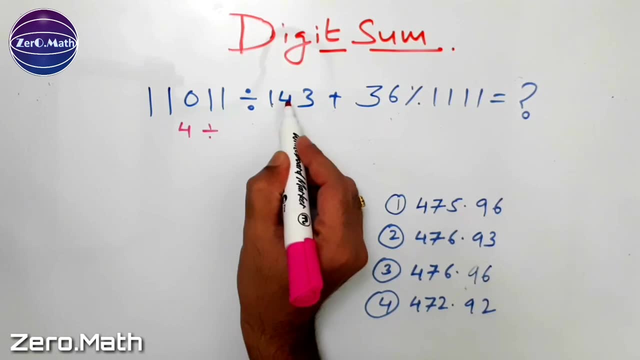 So division problems are a bit tricky, Let's understand how to solve them. So let's find out the digit sum 1, 1, 1, 1.. So it's 4 by 4 plus 1,, 5 plus 3, 8.. 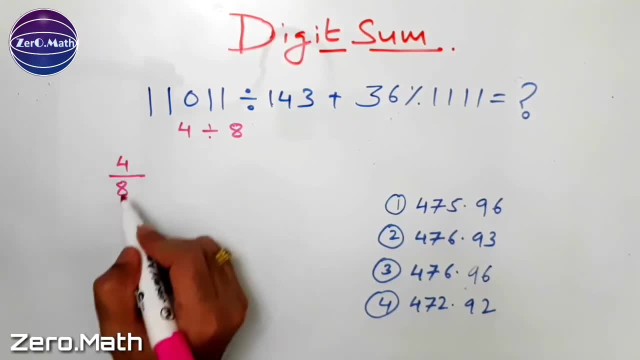 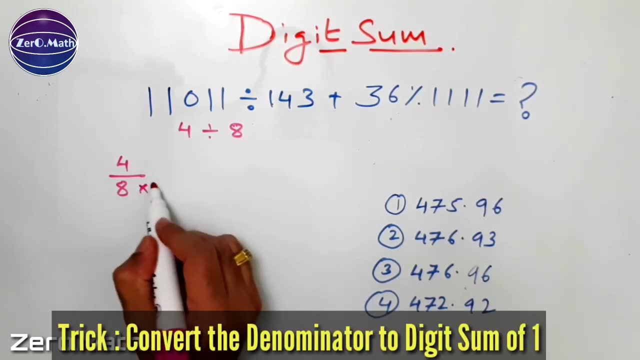 So the trick here is how to find out the digit sum of 4 by 8.. So what we are going to do, we are going to convert our denominator into the digit sum of 1.. So 8, if multiplied by 8, we'll get 64.. 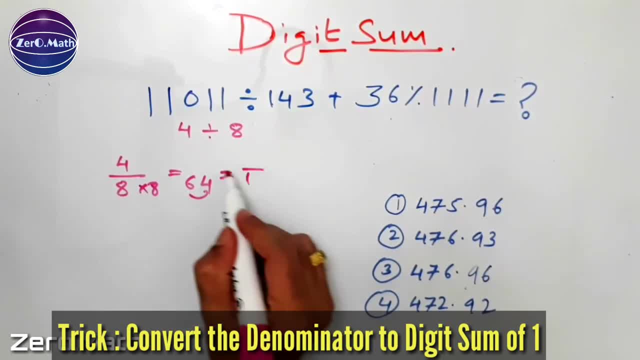 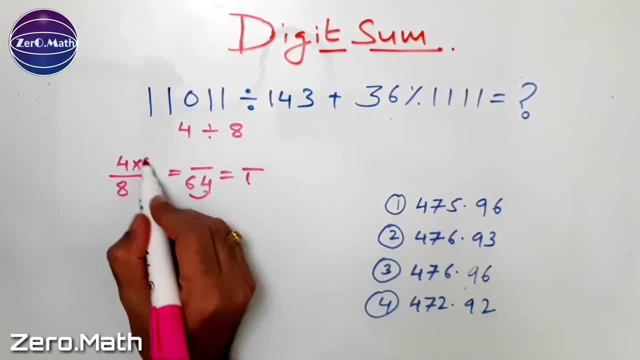 So 6 plus 4 is 10, which is 1.. So the digit sum of denominator will be 1.. So since I'm multiplying my denominator by 8, I will multiply my numerator also by 8.. 8 into 4 is 32.. 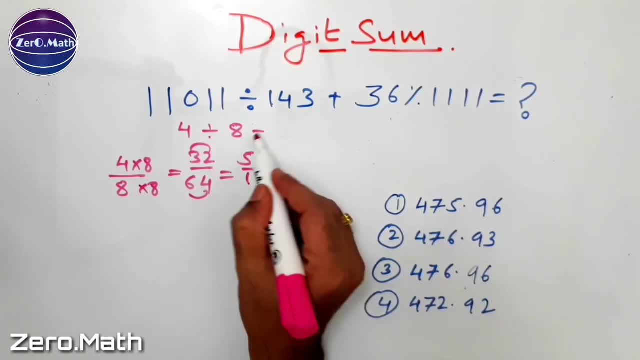 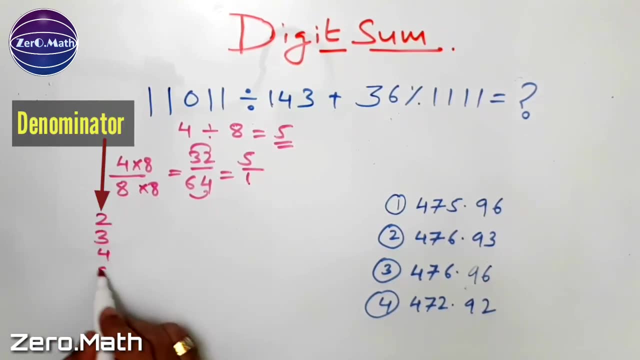 So 3 plus 2 is 5.. So 5 by 1 is 5,, which is my digit sum. So what if I have 2,, 3,, 4,, 5,, 6,, 7 or 8 at the denominator? 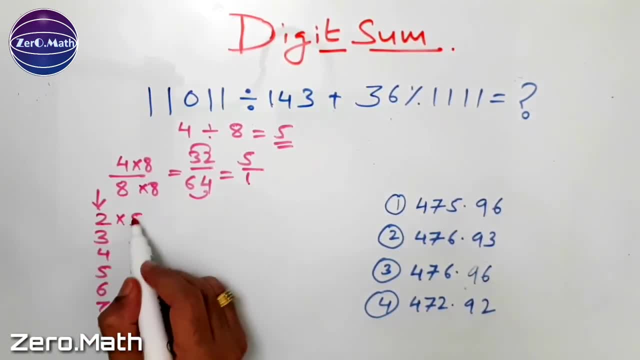 If I have 2 at the denominator, I'll multiply it by 5.. So 5 into 2 is 10.. So the digit sum of denominator will become 1.. So if I have 3 and 6, if you multiply 3 and 6 by anything, you will never get digit sum as 1.. 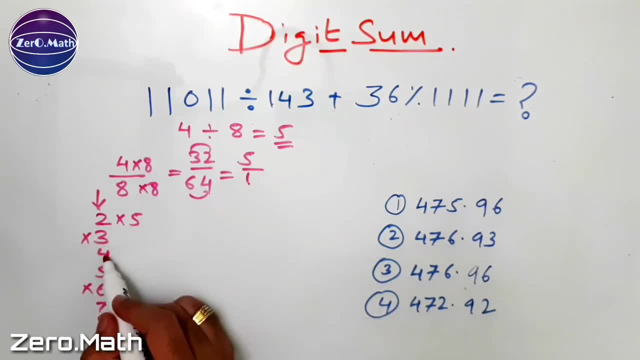 So you have to find out some alternative method in such cases. So if you have 4 in the denominator, you will multiply it by 7.. 7 into 4 is 28.. So the digit sum will become 1.. So if 5, you will multiply it by 2.. 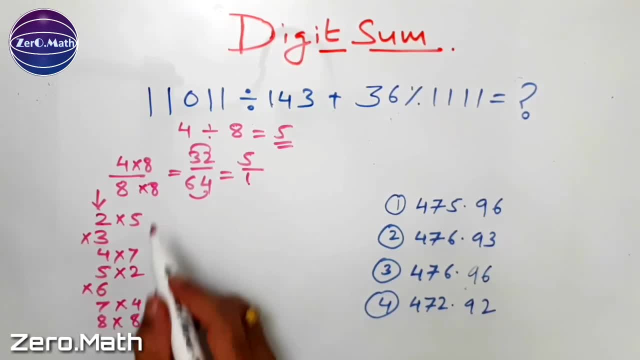 In case of 7,, you will multiply it by 4.. And in case of 8,, you will multiply it by 8.. What we have done here? So this You have to remember. Let's find out the digit sum here. 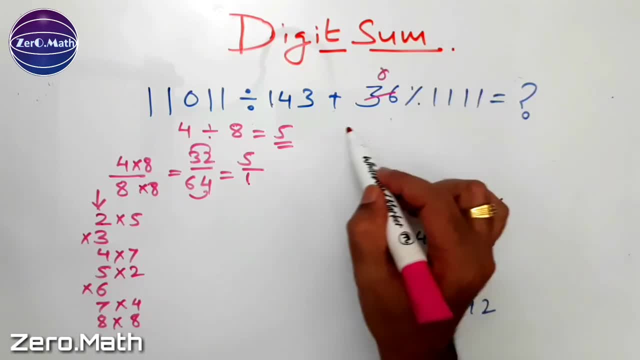 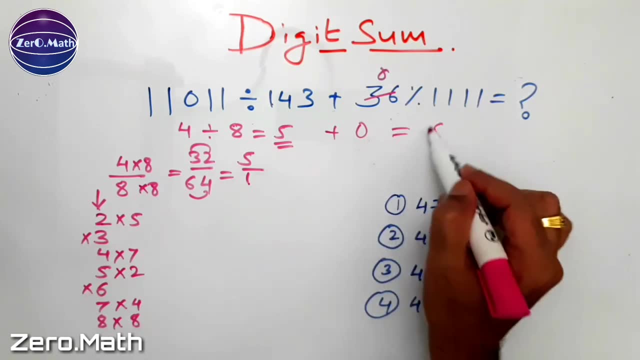 So 6 plus 3, 9.. So it will become 0.. So, anyway, the digit sum of this part, 36% of 1, 1, 1, 1- will be 0. So 5 plus 0 is equal to 5,, which is my digit sum of right hand side, which has to be my digit sum of right hand side. 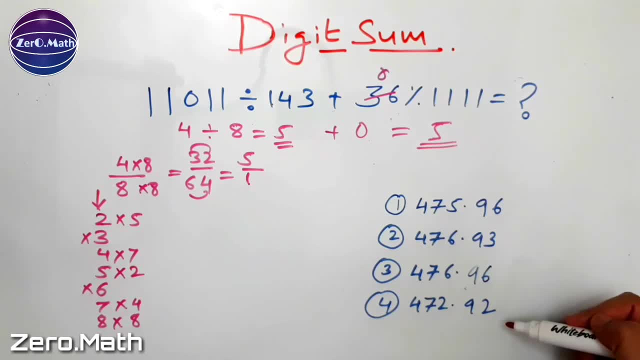 Let's figure out of these four options which option has digit sum as 5.. Take the first option: this: 9 gone, 6 plus 5, 11.. 11 plus 7 is 18 plus 4, 22.. 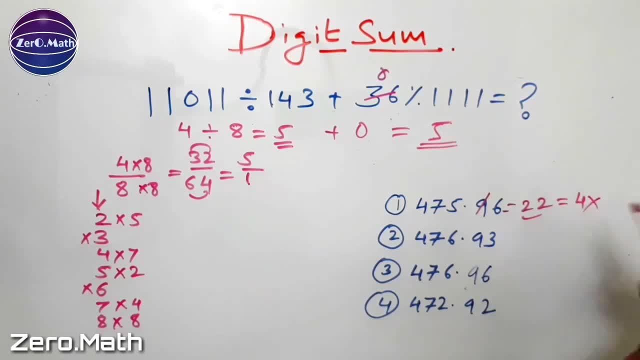 So the digit sum of 22 is 4.. This cannot be the answer. Let's take the another option, 2.. So 9 gone, 6, 3, 9 gone, 7 plus 4, 11, 1 plus 1, 2.. 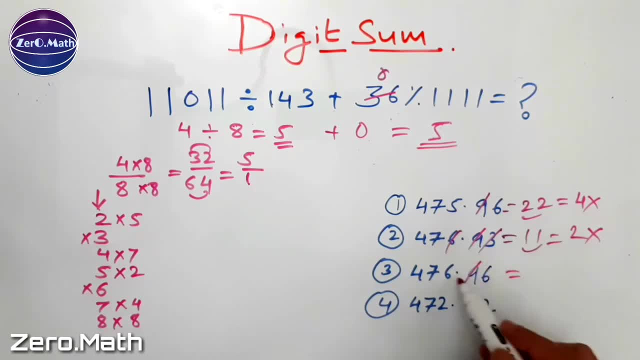 This cannot be. Let's take third one. So this 9 gone, 6, 6, 12.. 12 plus 7 is 19 plus 4, 23. So 2 plus 3 is 5.. So yes. 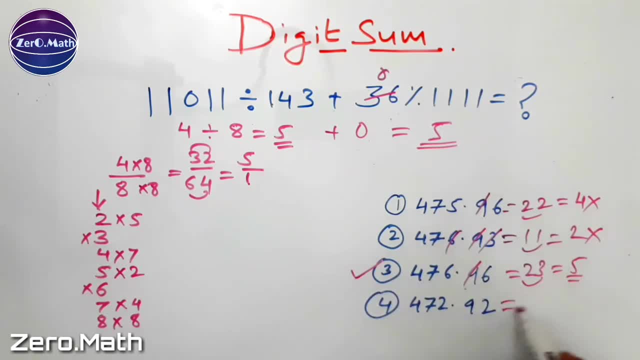 The digit sum is valid. The digit sum is matching, So this can be my answer. Let's try the last option: 9 gone 7, 2, 9 gone 0. So 4 plus 2, 6.. 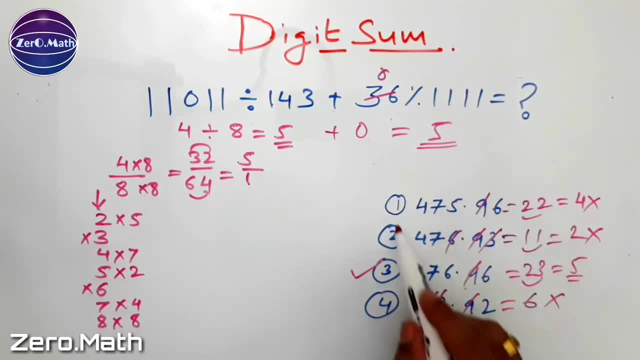 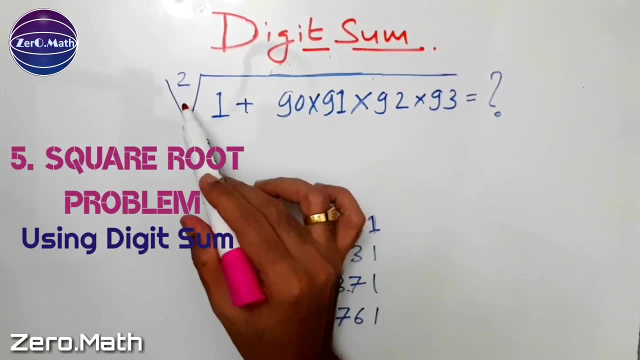 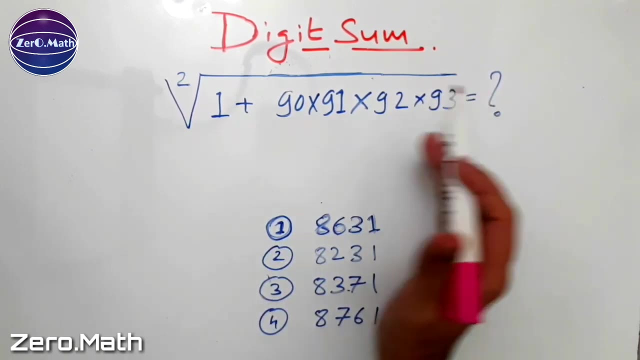 This cannot be my answer, So the answer is option 3.. Let's solve this square root problem using the digit sum method. This is a famous problem asked in many competitive exams, So pay your attention. Let's find out the digit sum of left hand side. 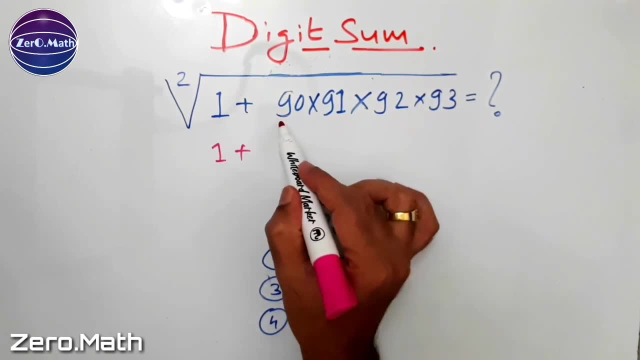 So it's 1.. It's 1.. It's 1.. This is 10.. This is 10.. It's 20.. This is 13.. This is 14.. This is 15.. This is 16.. 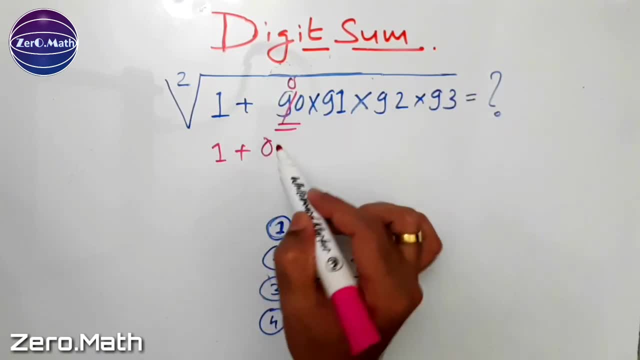 This is 17.. And this is 20.. So it connects to 0.. And this is 20.. This is 22.. This is 21.. This is 52.. And this is box one. This is two, So we have done about 20.. 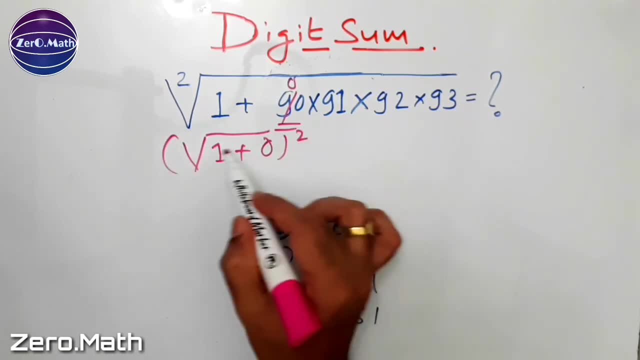 This is a maximum, infinite digit sum. This is aqualite. I am going to take a square root of this square root. So, in that case, what we will do? We will take square of this figure, So, square root of one, we will get one. 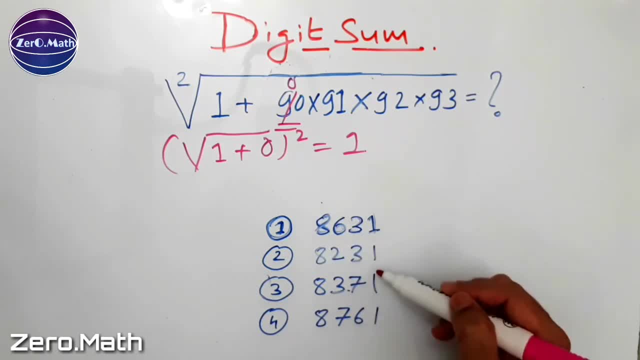 Since we have taken square here what we are going to do, We will take a digit sum of each of this option. So this is an important step and most of the students do mistake over here, So be careful about it. Let's find out: digit sum of option 1.. 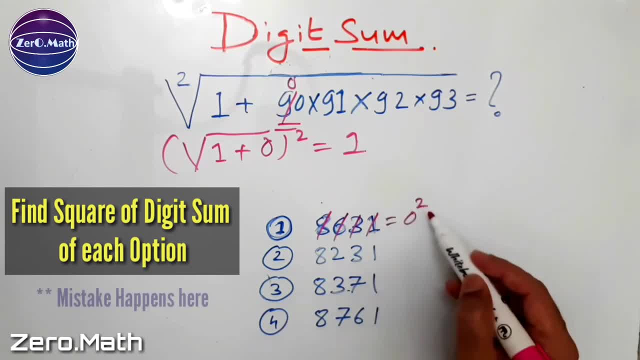 8 and 1, 9 gone. 6, 3, 9 gone, So it is 0.. 0 square is 0.. This cannot be our answer. Take second option: 8, 1, 9 gone. 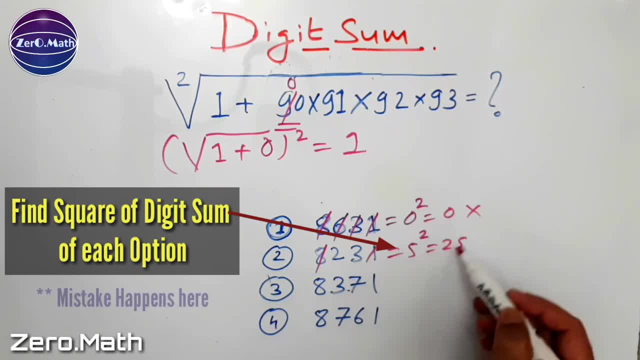 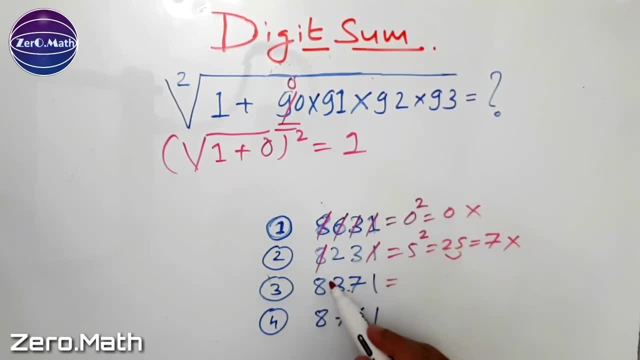 2 plus 3, 5.. Take square of 5, which is 25.. And 25 means 5 plus 2, 7.. So this cannot be our answer. The digit sum has to be 1.. Take the third option. 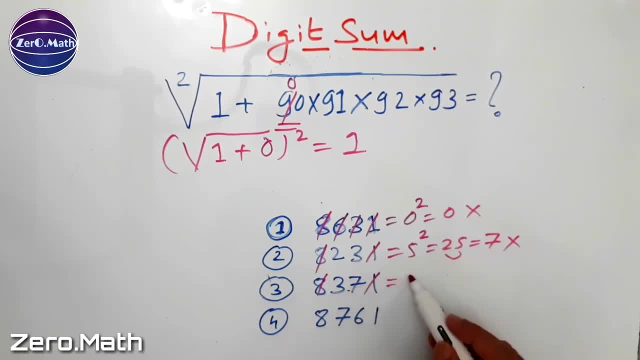 8, 1, 9 means 0.. 7 plus 3, 10.. So 10,. the digit sum is 1.. So take square of 1.. 1 square is 1.. So yes, this can be our answer. 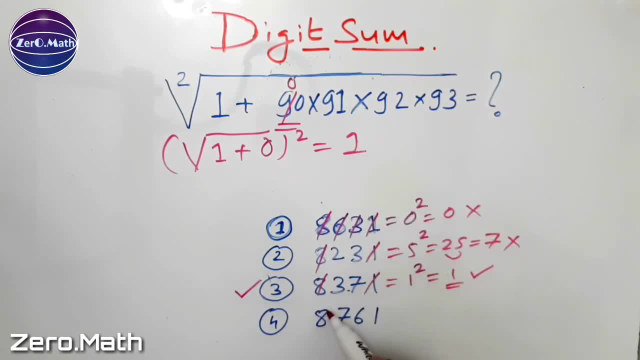 However, let's find out the digit sum of last option: 8 and 1,, 9 gone, 7 plus 6,, 13.. 13 means 3 plus 1,, 4.. Digit sum is 4.. Take square of 4.. 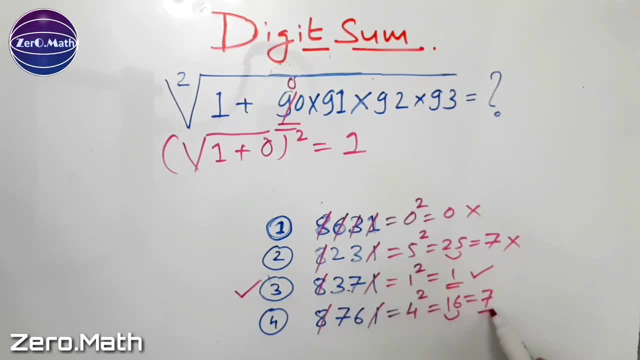 4 square is 16.. So 6 plus 1 is 7, which cannot be our answer. So our answer is option 3.. So you can see this problem, even though it looks complicated. using the digit sum method, We can find out the result very quickly. 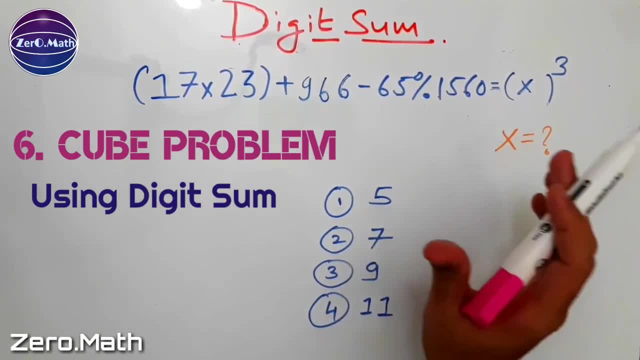 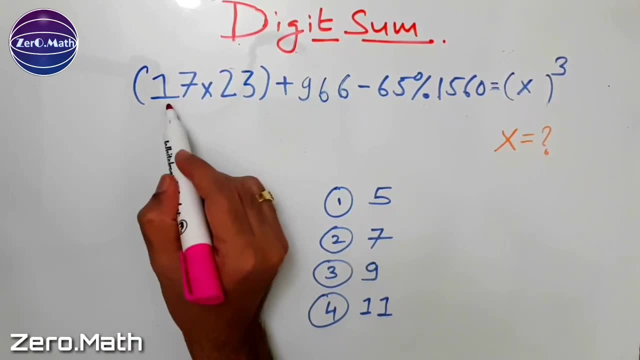 Let's solve this final example along with me as a practice session. Find out what is the value of x from these four options. So let's take a digit sum of left hand side, So it's 7 plus 1, 8.. 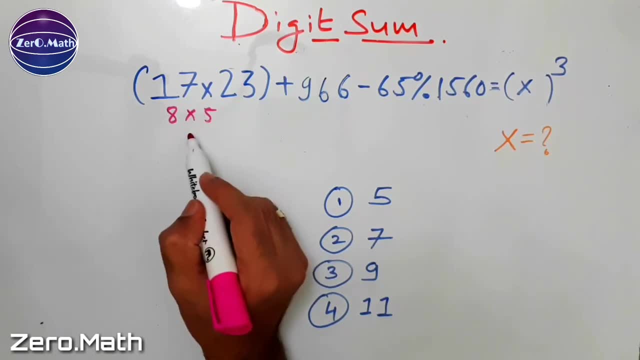 8.. 2 plus 3, 5. 8 into 5 is 40. So 4 plus 0 is 4.. Plus this is 9 gone. 9 means 0.. 6,, 6,, 12.. 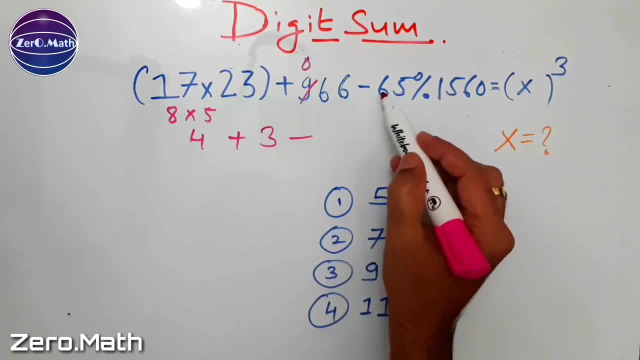 So 12 is 2 plus 1, 3.. Minus 65.. So 65 means 6, 5, 11.. So 11 is 1 plus 1, 2.. Percentage means into 1,, 5, 6, 0.. 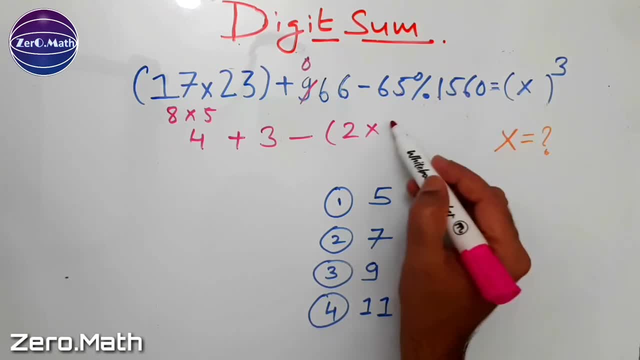 So 6, 1, 7 and 5, 12.. So 12 means 2 plus 1, 3.. So 4 plus 3.. 7 minus 6 is equal to 1.. So pay your attention here. 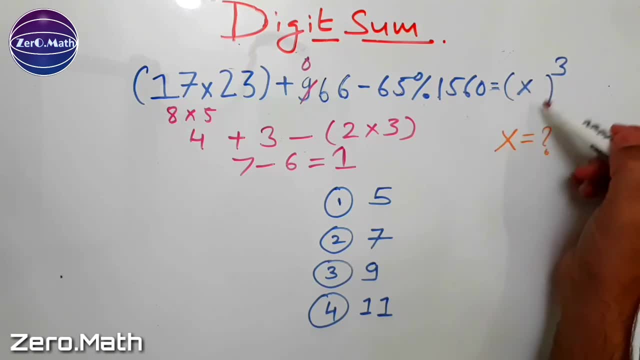 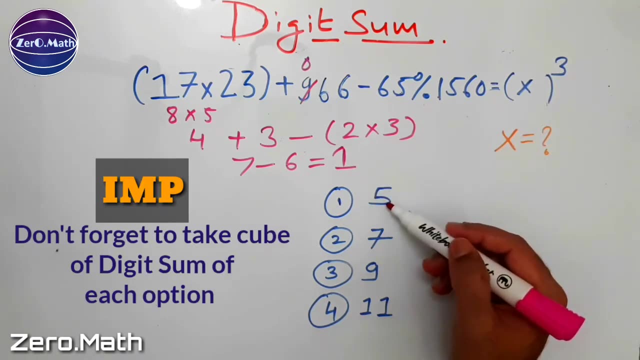 So digit sum of x, if we take cube of that figure, that should equal to 1.. So basically what we are going to do for each option, we will find out the digit sum and we will take a cube that should match with 1.. 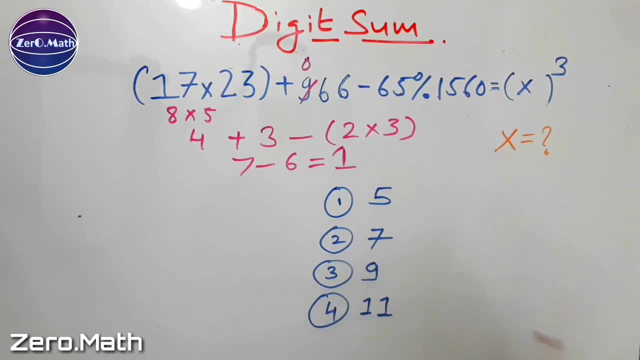 So whatever option matches, that is our answer. So take the first option, 5.. So 5 cube is 125.. So it is 5 plus 2, 7 plus 1, 8.. So this cannot be our answer. 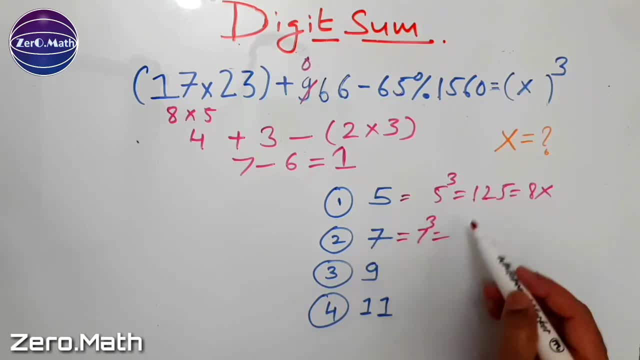 7.. So what is the cube of 7? 343.. So 4 and 3, 7. Plus 3, 10.. So 10 means 1.. 1 plus 0 is 1.. So yes, 7 can be our answer.